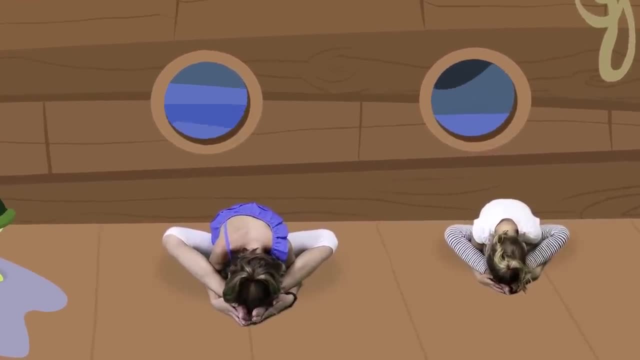 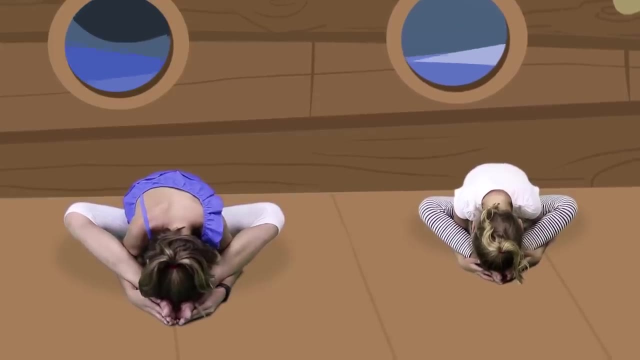 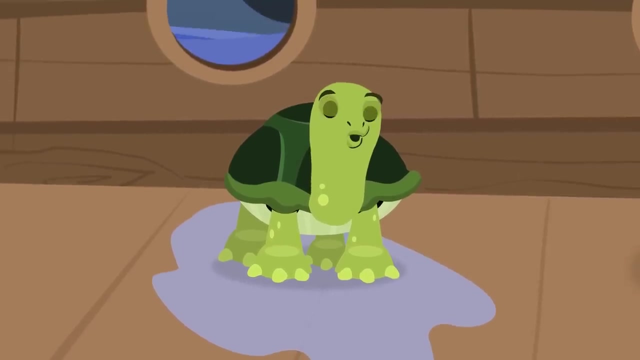 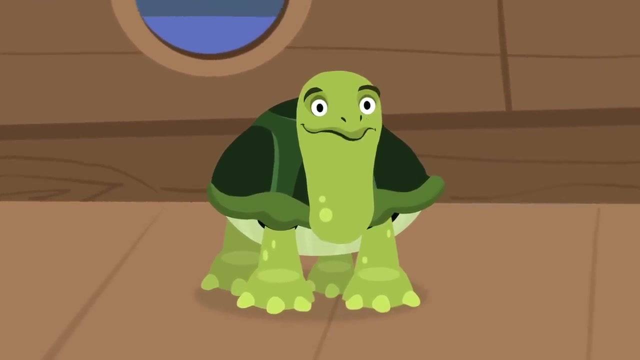 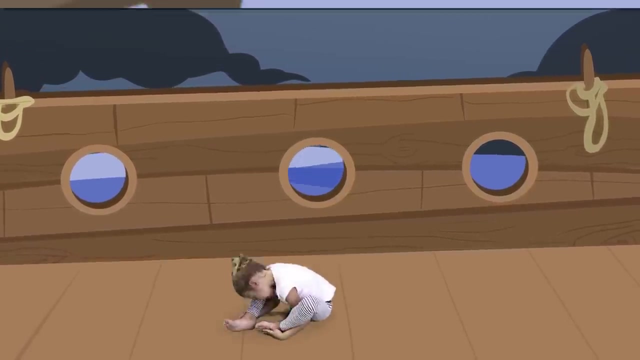 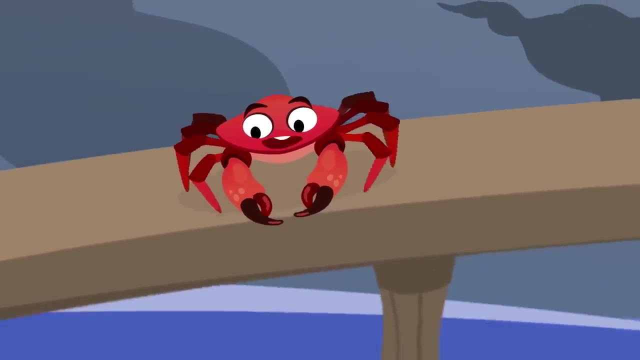 Can you feel how your back is curved, just like a turtle shell? Try to keep the pose for at least one minute. And this is the turtle pose. I think I'll swim back to the sea. Hey there, I see you're doing yoga. Would you like me to show you the crab pose? Let's give it a go. 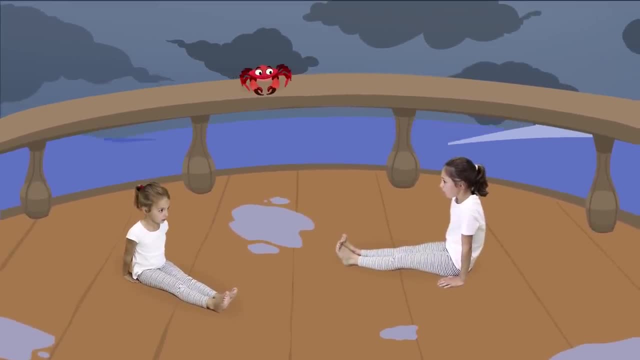 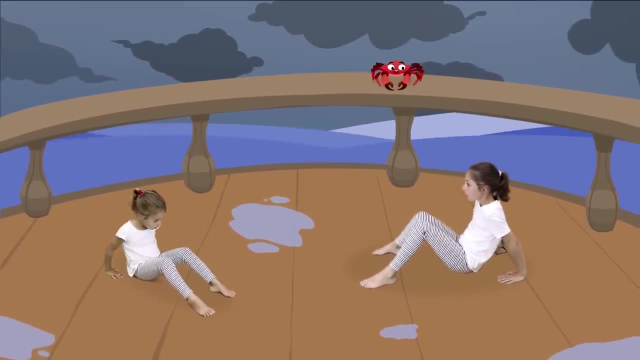 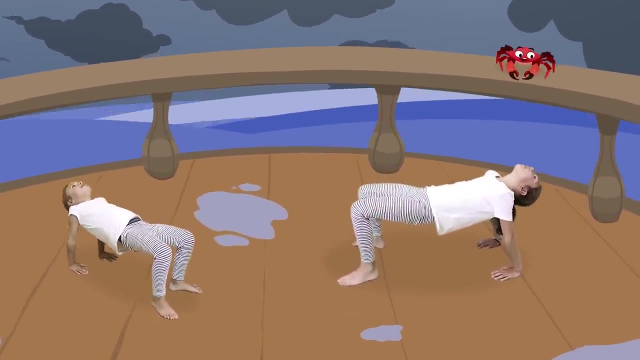 Sit on the floor and flex your knees. Keep your feet firmly on the ground and bring your palms next to your wrists. Inhale and lift your hips. torso and head- Your body now looks like a box. Look up and keep the pose. 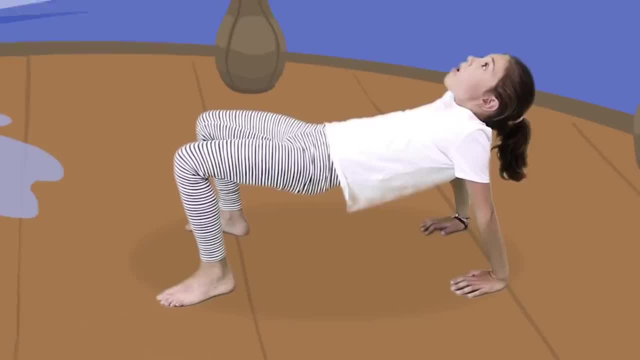 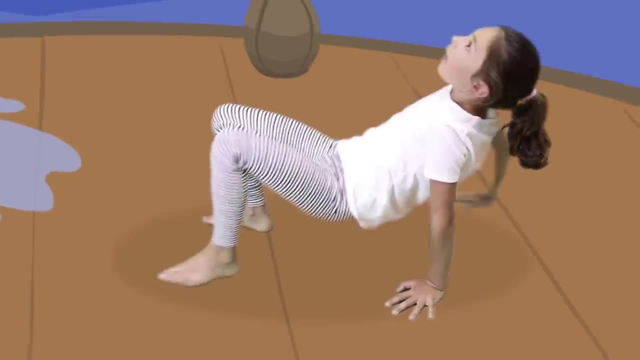 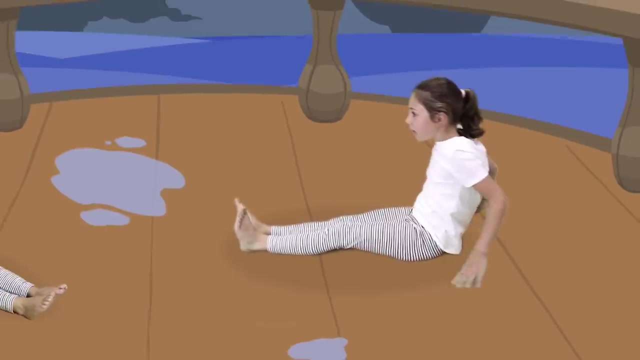 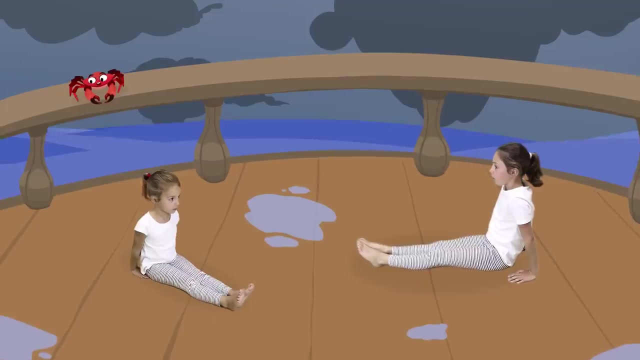 for five seconds. Try walking like a crab, just like me. Move forwards and backwards. Well done. Now exhale and sit on the floor again, Rest a little and repeat the pose at least five times. The crab pose is really awesome, isn't it? 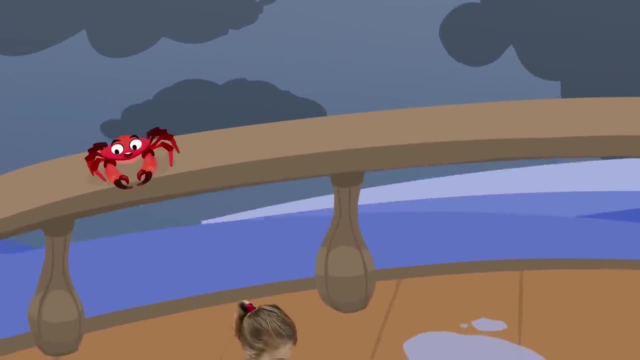 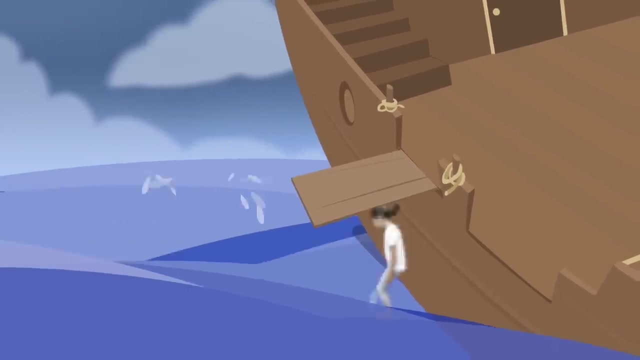 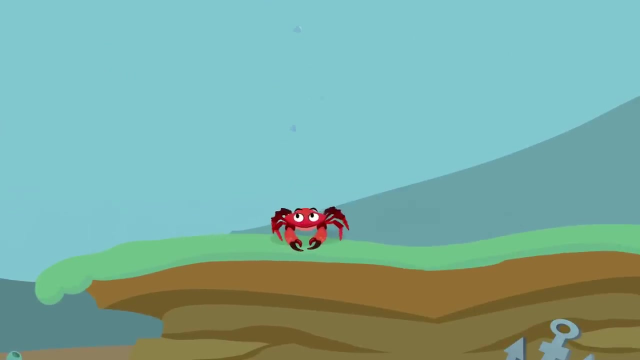 Would you like to learn more poses? Come with me then, deep in the sea. I have many friends there who can help you. This is my friend the shark. Hey friend, Don't worry, I'm a good shark. I'm going to show you the shark pose. 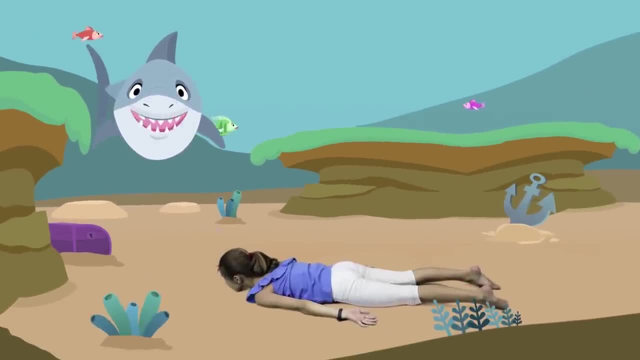 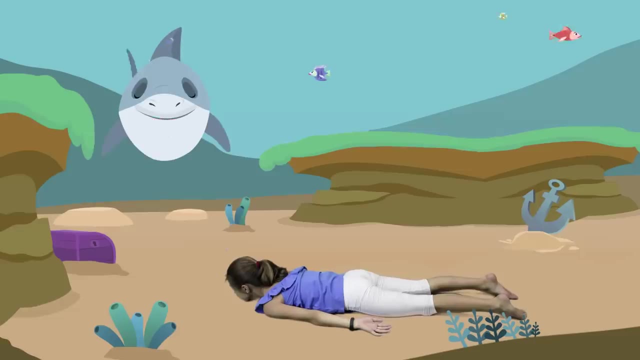 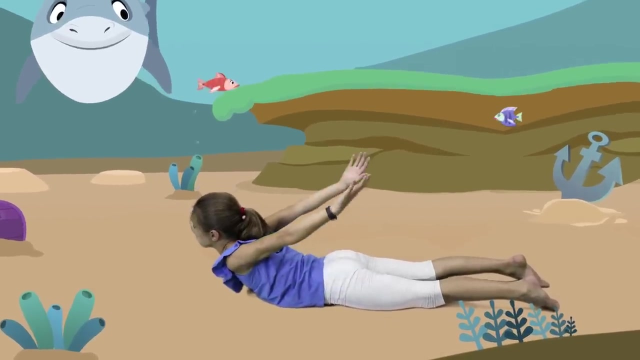 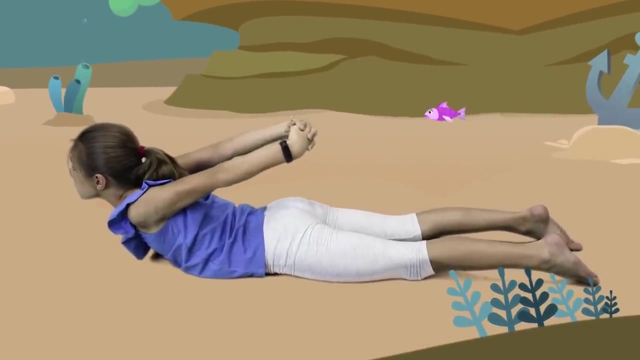 Lie down on your belly and place your arms on each side of your body. Your palms should be facing upwards. Look up, inhale and raise your head, shoulders and ribs. Bring your hands and palms together and crisscross your fingers behind your back, making a shark fit. 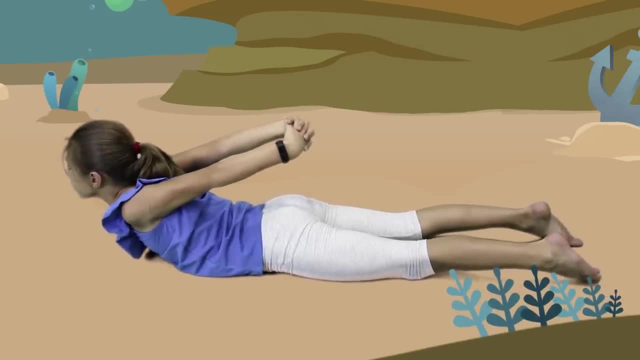 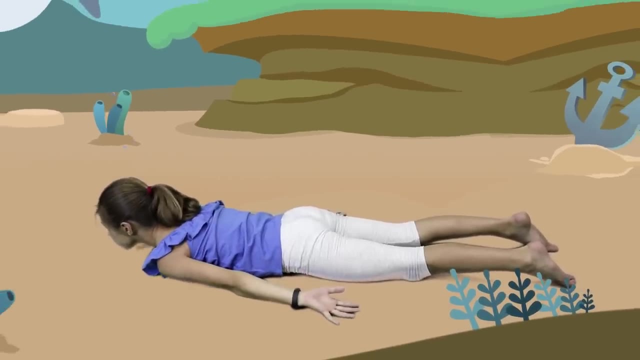 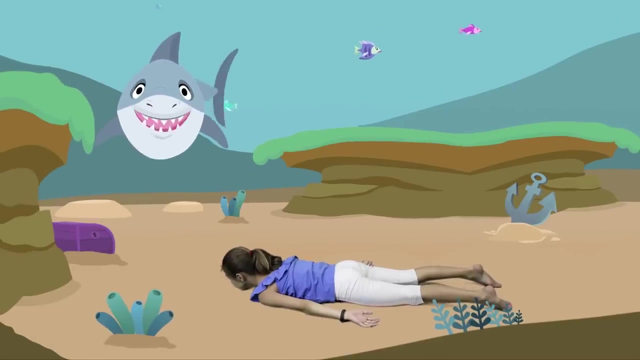 Keep the pose for five seconds, Exhale, Bring your hands to the initial position and come down. Repeat the pose at least five times. Amazing, You did so well. I think I can see my friend the starfish over there.